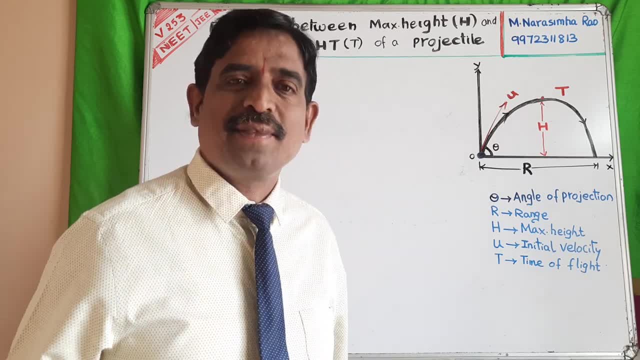 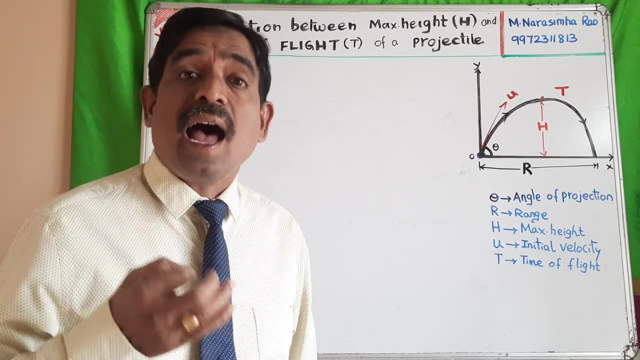 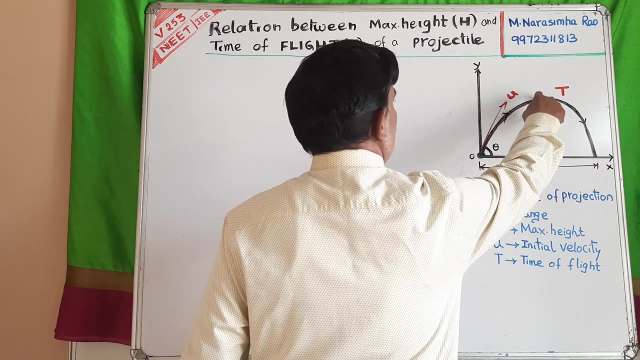 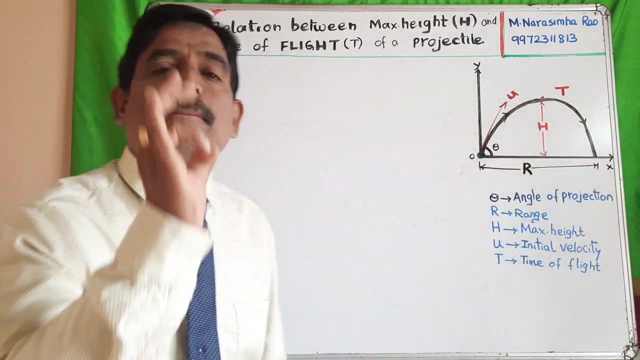 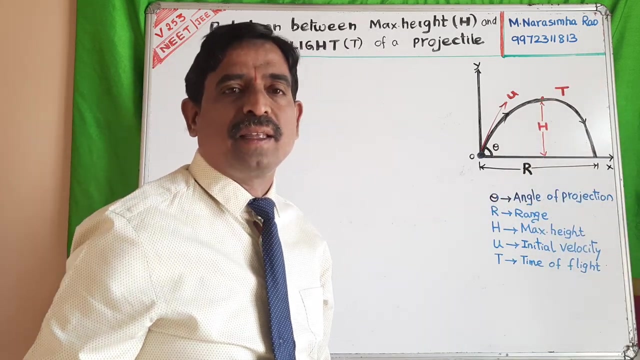 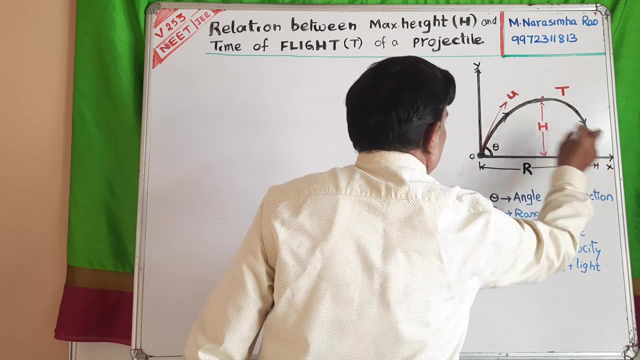 My name is M Narasimha Rao, lecturer in Physics. Today I am explaining relation between maximum height of the projectile and time of flight of the projectile. Best example for projectile is ball hit by the batsman. The total time for which the projectile is staying in air. 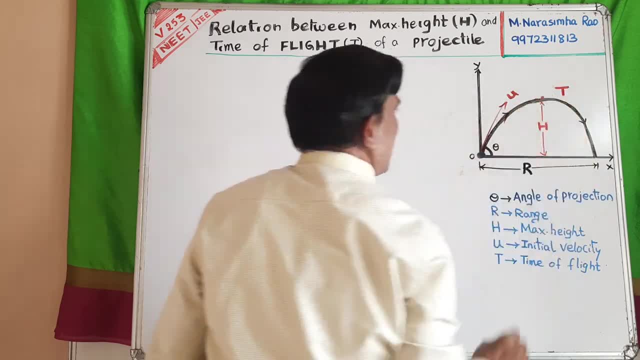 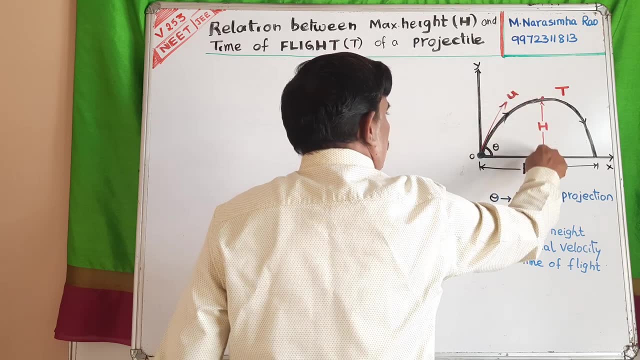 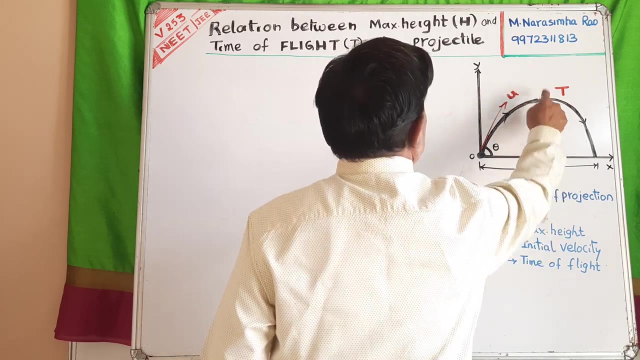 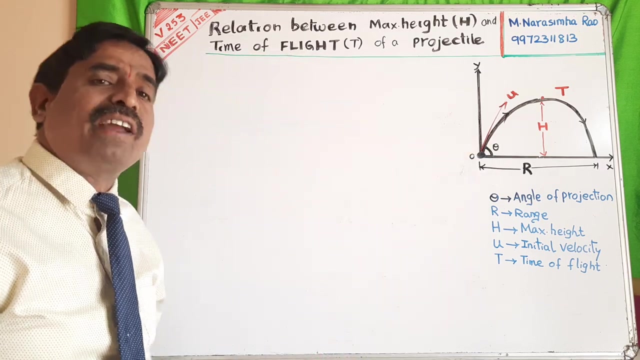 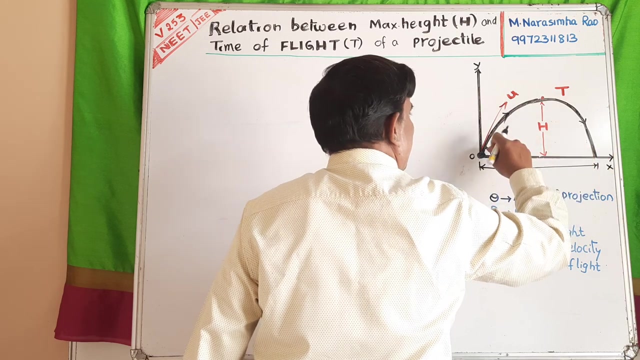 this total time. we are calling as time of flight The maximum vertical displacement of the projectile above the horizontal level. we are calling as maximum height Here theta is the angle of projection. We are having one formula for time of flight: the total time for which the projectile is staying in air. Time of flight, formula time. 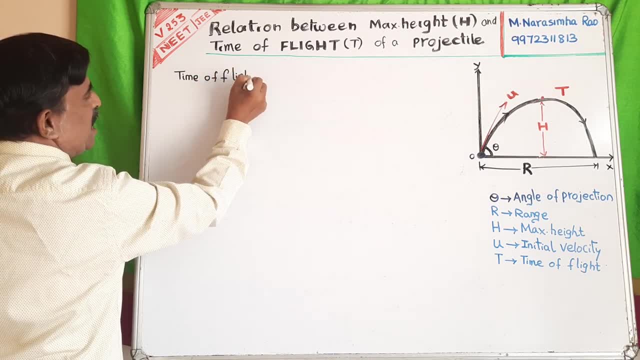 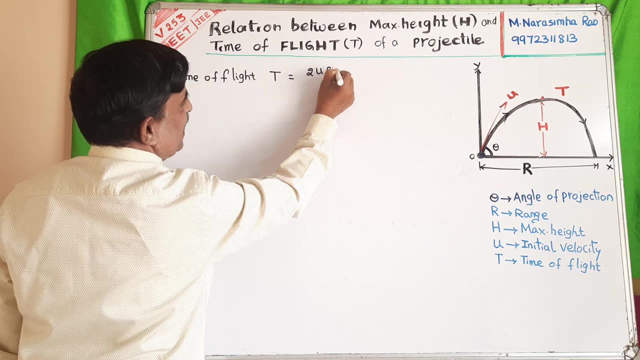 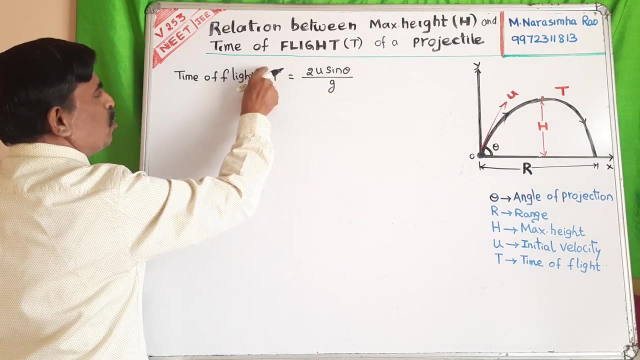 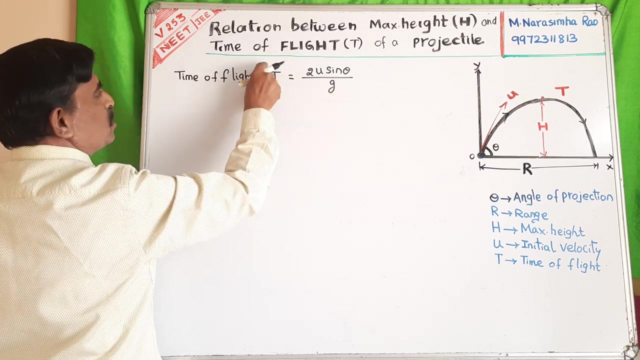 of flight. formula: time of flight. t is equals to 2u sin theta divided by theta. This is the equation of theta divided by g. Now please listen here. g comes to numerator g comes to numerator. 2 comes to denominator. g comes to numerator g. into t, g into t. gt by 2 comes. 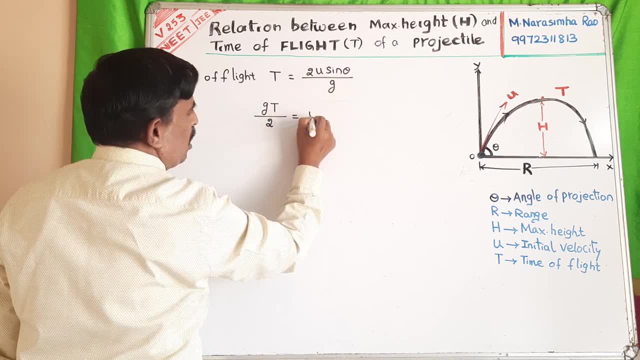 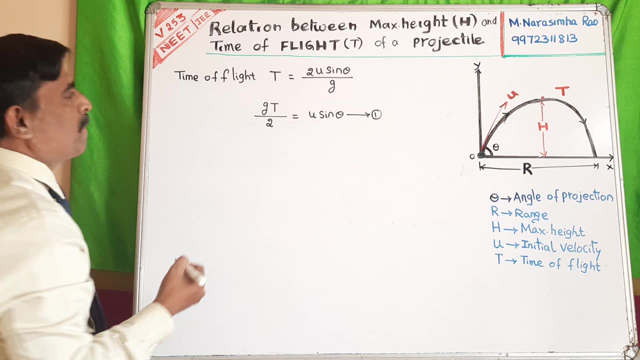 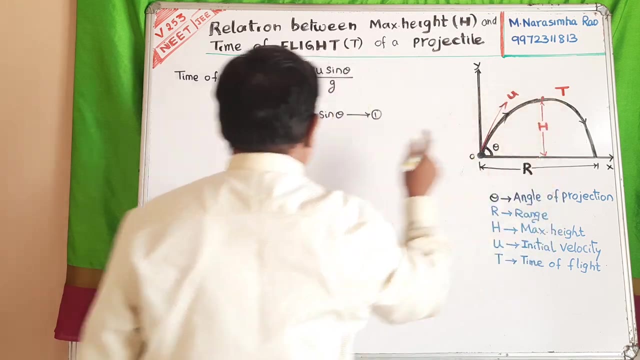 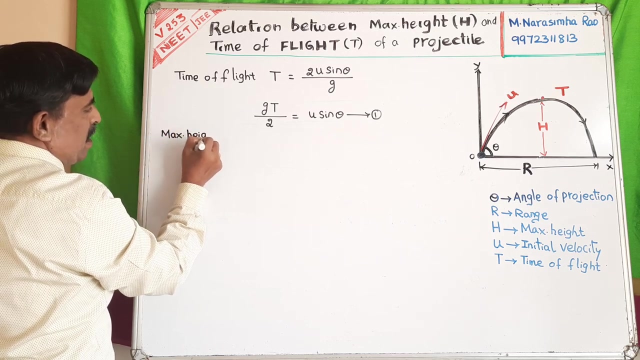 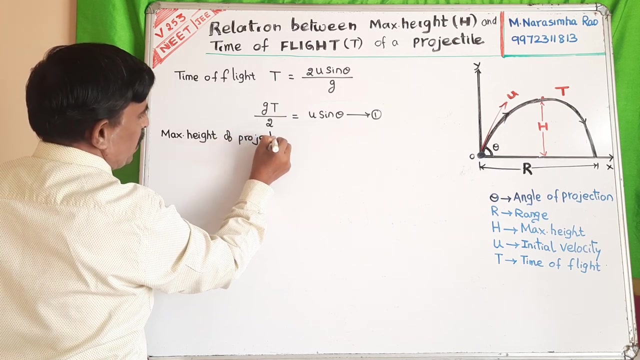 to denominator. That is equals to u sin theta. It is equation of theta divided by theta. Now we are taking the number of the projectile. Now if I want the height of the projectile, we have to say that hc is equal to u square minus theta. So we are taking the height. 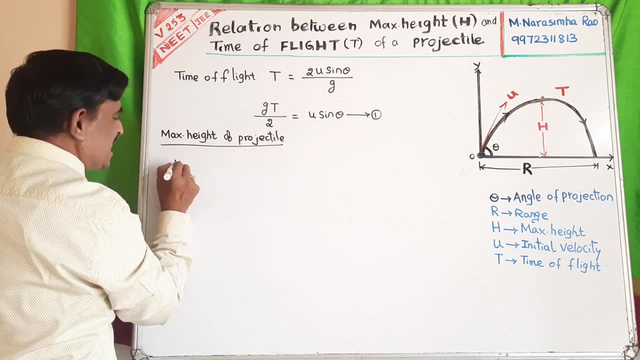 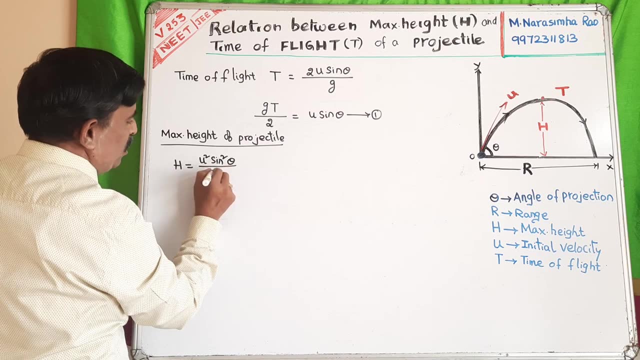 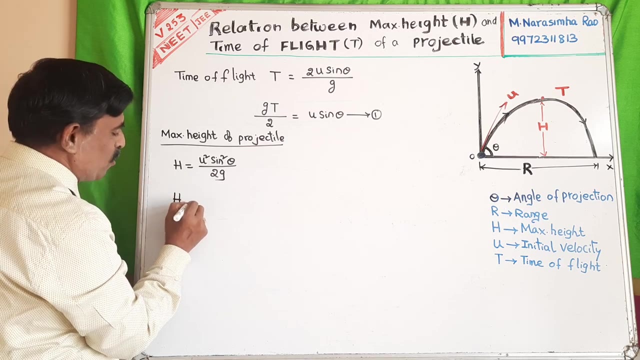 of the projectile. we are taking the height of the projection. This is the equation of height of the projectile: 1. sine square theta by 2g. Now this can be written as: h is equal to u square sine square theta.